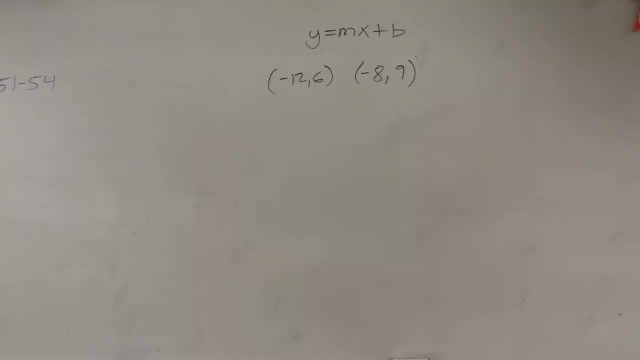 That you could probably easily do with point-slope form again. Alright, that form over there. However, I think a lot of you understand this method, so let's just work with it. So we don't know what the slope is. 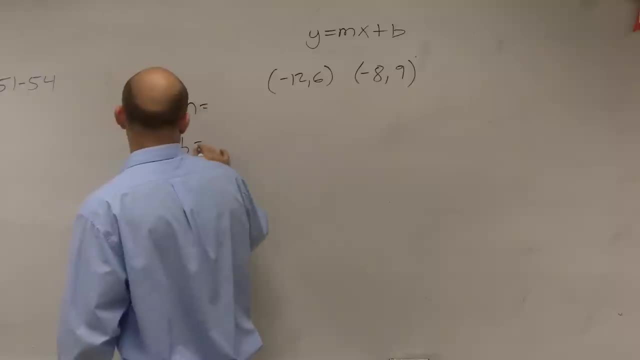 All we need to do to solve this equation, or to find the equation, is to find out what m is and what b is right. So we're given two points. So how do we find out what m is? Well, we have to go back to our slope form. 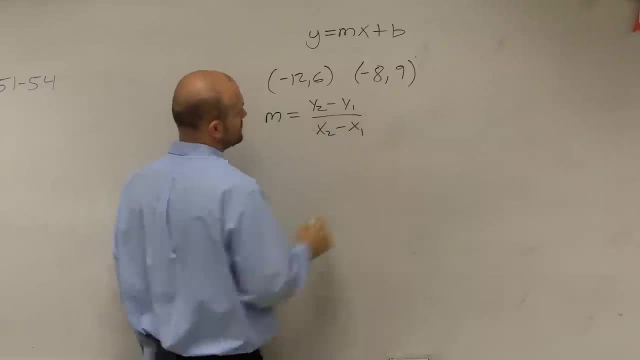 which is y2 minus y1 over x2 minus x1.. Right, So then we label these. Which one's x1, which one's x2? It doesn't matter. Do we know that's an x and that's an x? 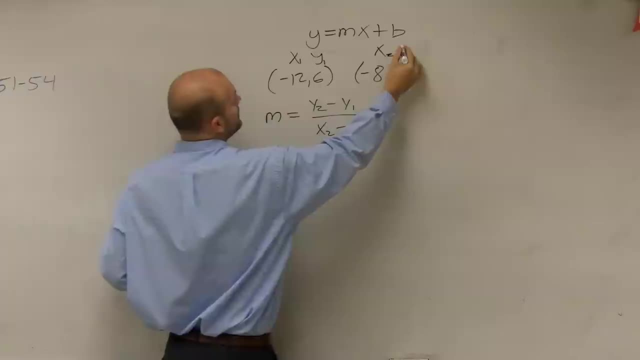 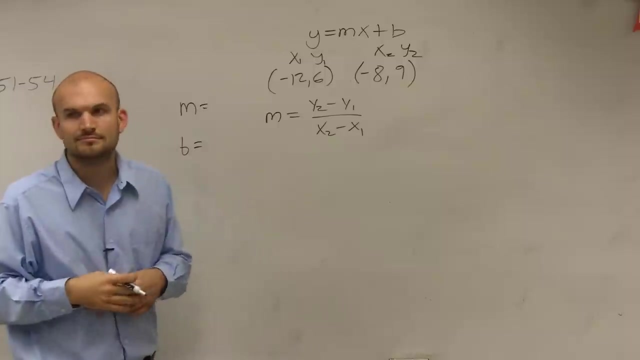 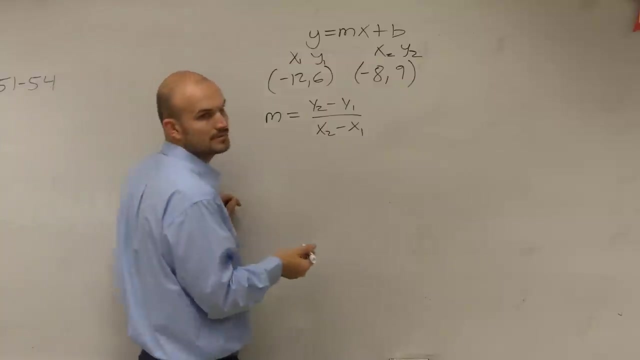 Pick one to be 1,. pick the other to be 2.. y1, y2.. Yeah, as long as you're consistent, it doesn't matter. Okay, Just make sure you're consistent. y2 minus y1.. x2 minus x1.. 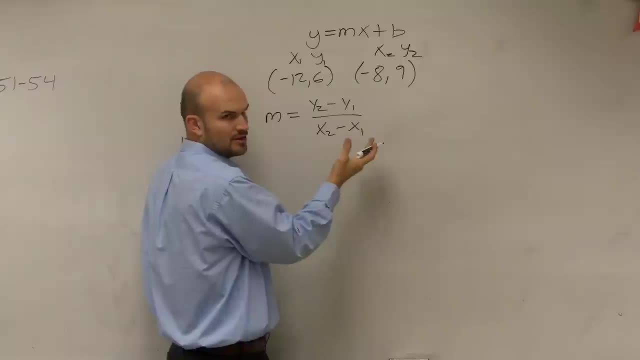 Don't do y2 minus y1, and then do x1 minus x2.. You know what I'm saying. Just be consistent and you're fine. So 9 minus 6 over negative 8 minus a negative 12.. 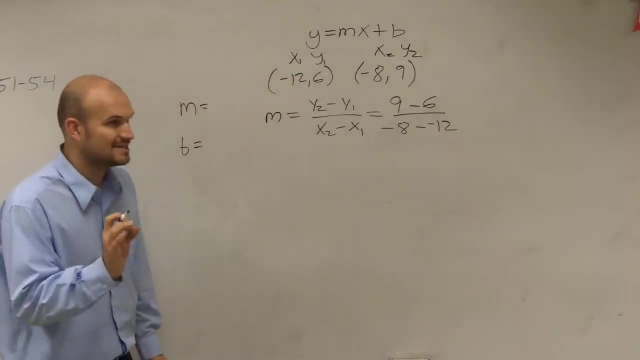 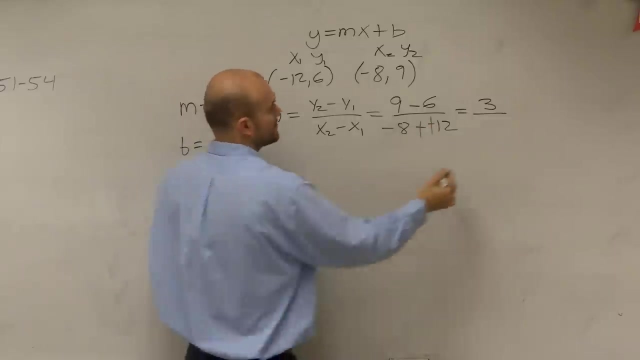 Right Negative 8 minus a negative 12. Right, You guys have to be very careful when you do this. So 9 minus 6 is 3.. 8 minus 8 minus a double negative is now going to be 4.. 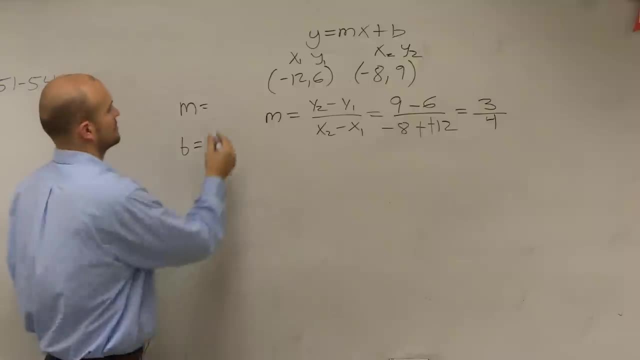 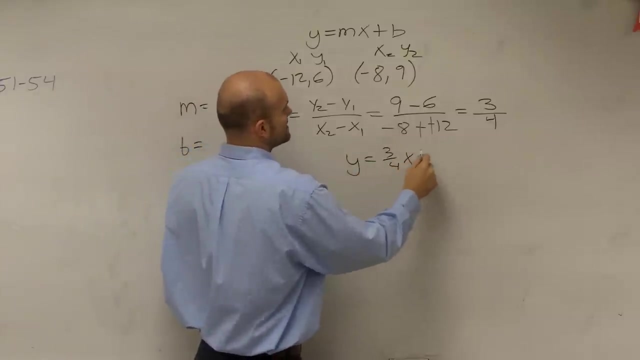 Okay, So now do we know what slope is? So we're halfway there Now. so we write our equation: y equals 3 fourths x plus b, But we still don't know what the y-intercept is. So what's the only piece of information that we're given, Trevor? 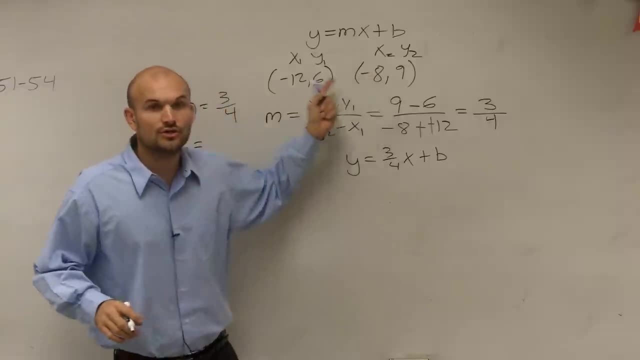 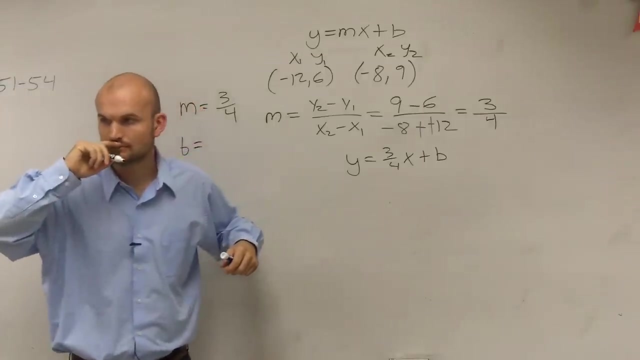 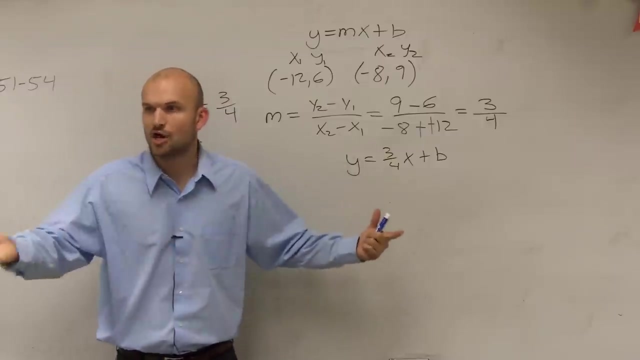 Well, we're not given slope. We just found out slope. But we are given two points And remember the last problem. Yes, Chase, Yeah, because that's what we did in the last problem. right, We took the points and we plugged it in for x and y to solve for b. 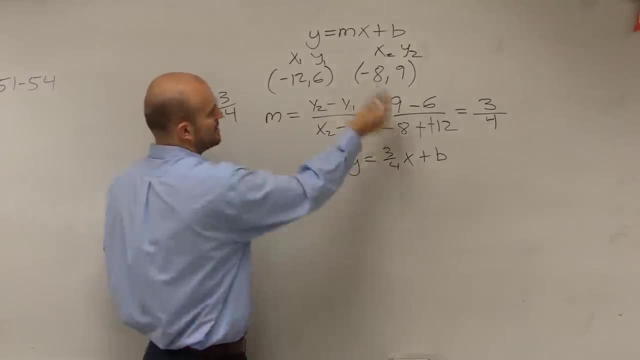 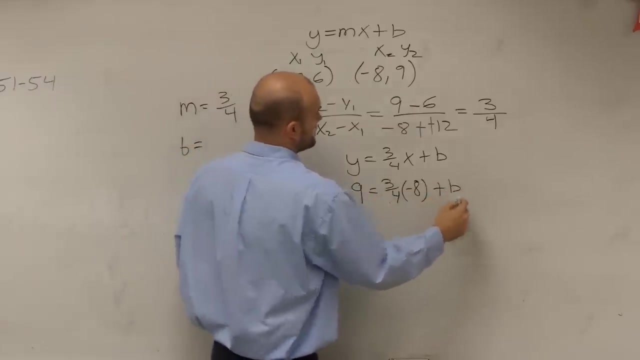 So let's just pick a point. Which one do you guys want to do? Any, All right, let's do the. I'll do this one. I kind of like this one. 9 equals, It does not matter. And if you guys want to do the other one on your own.